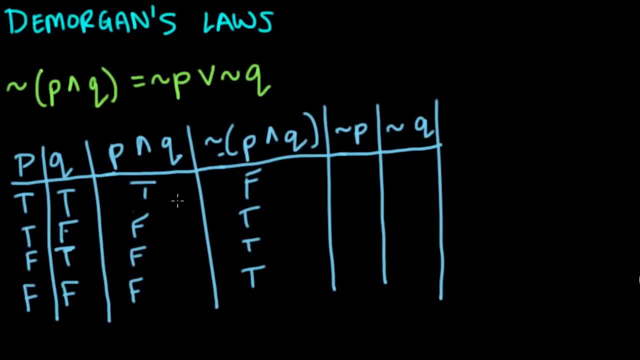 not q. so basically now we're going to reverse these signs. so we have false, false, true and true. i'm just reversing these one, two, three, four there, and the same thing with the q. we're going to reverse them. so whenever it's true becomes false. whenever it's false, it becomes true, right? so we? 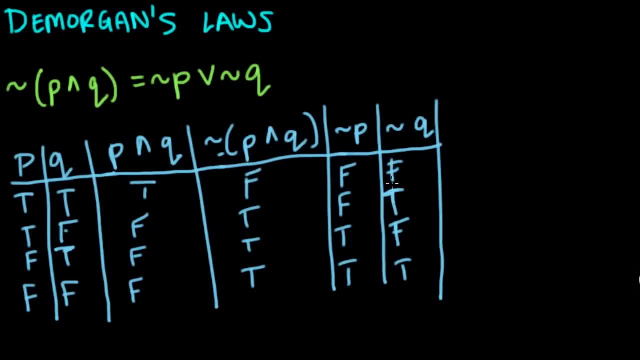 have and- sorry, my handwriting is a little sloppy- i realize we have false true, false true. so now we have not p or not Q. That's what we're finding. So if we're correct here- and this is why there's no need to memorize- we should get the exact. 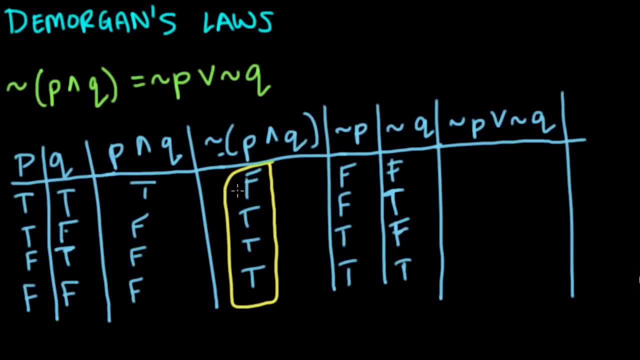 same thing that we get here, because if they're logically equivalent, they'll give us the same output of false and true. If they're not, if it's not correct, if we made a mistake somewhere, often students forget: Is it or or is it? and 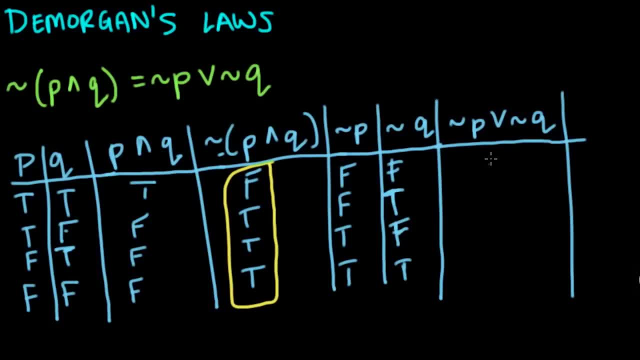 Which one do we do? I can't remember it? Well, plug it into the table here and see which one works. So here let's plug this in. So first we have an or statement to deal with And first we have two false statements. 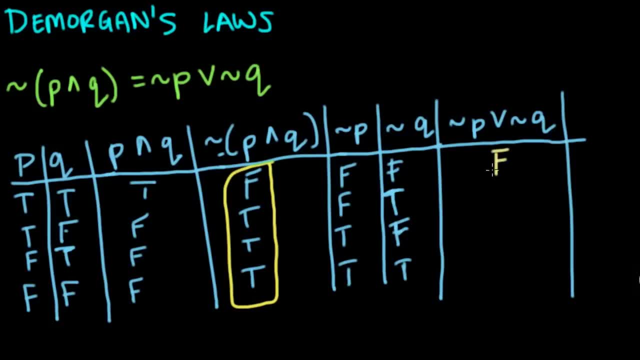 That means when you have an or statement and they're both false, it's still false. If one of them is true, it's true. False, true, True, false is true. And then, lastly, true or true is true. 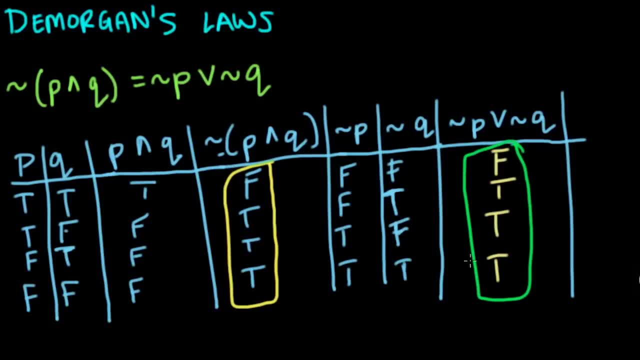 So here we get false, and then true, true, true, Which is equivalent to this statement right here. So these two things are equal. That's the first part of De Morgan's Law, And the second part follows a similar idea. The second part just says, okay, well, what if? 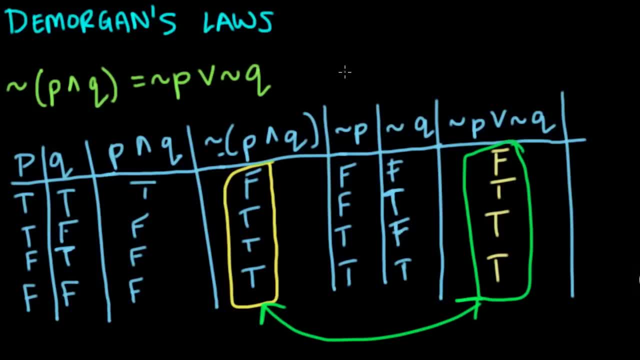 we're negating. let's negate p or q. What's going to happen? As you might predict, a very similar thing will happen here. We negate p and get not p. We negate the or sign and we get n. Then we negate q and we get not q. 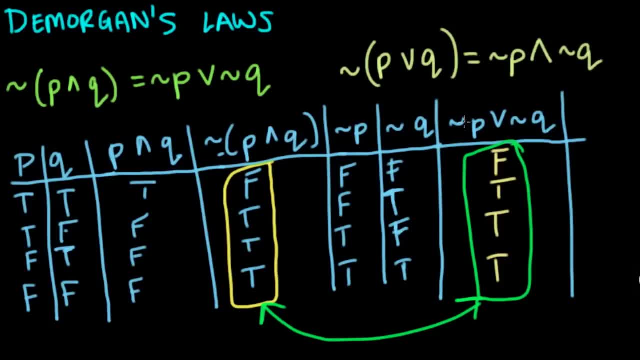 And if we don't believe that this is true, we can set up a truth table to test the validity. So let's do that real quick Because, like I said, I really believe there's no need to memorize any of this here. 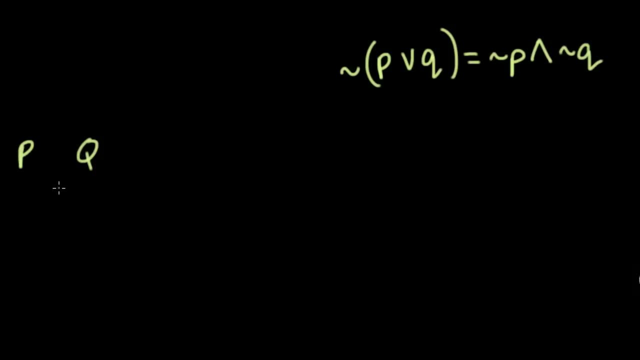 So again, we start with p and q, Although I should do lowercase q, because that's what I'm writing up here. So p could be true, and so could q. We could have true and false. We could have false and true, Or both terms could be false.